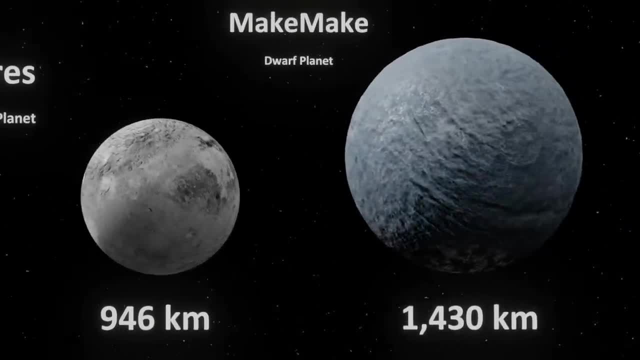 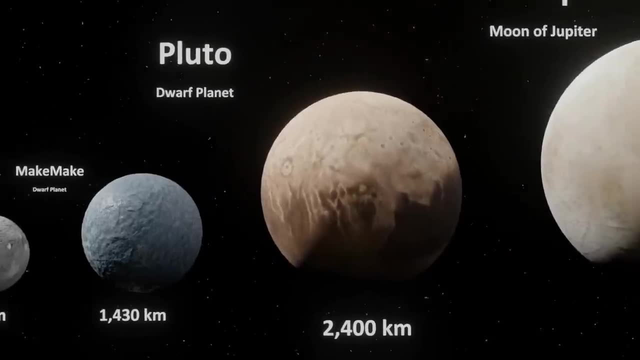 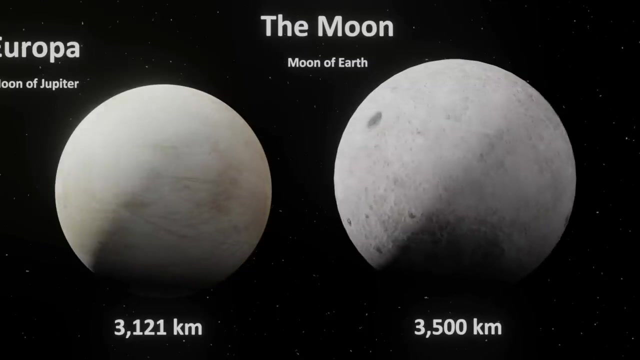 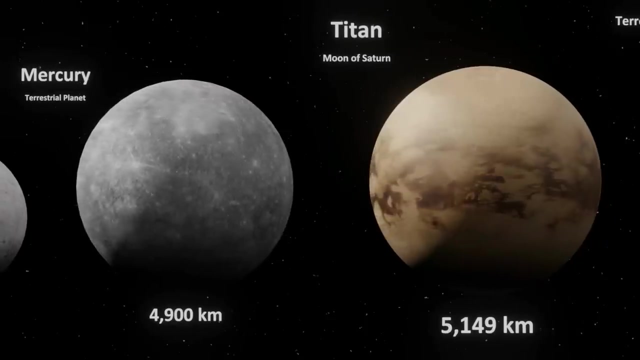 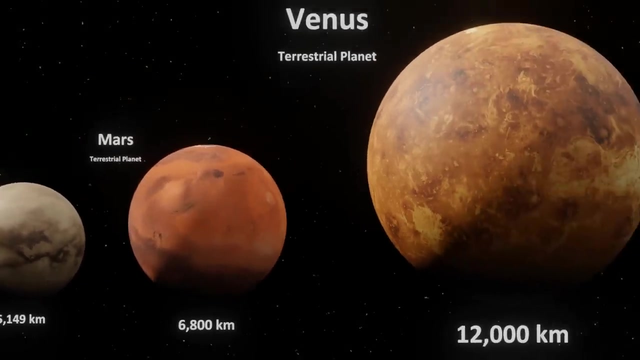 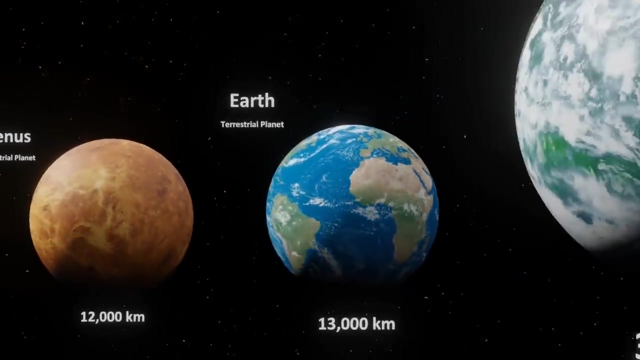 Please subscribe to the channel and press the bell to receive notifications when I upload a new video. Thank you very much for watching. Thank you very much for watching. Please subscribe to the channel and press the bell to receive notifications when I upload a new video. 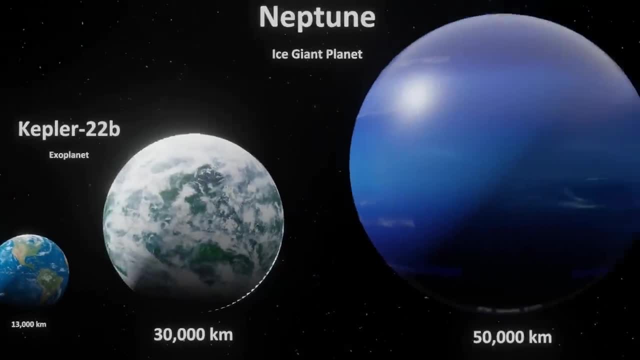 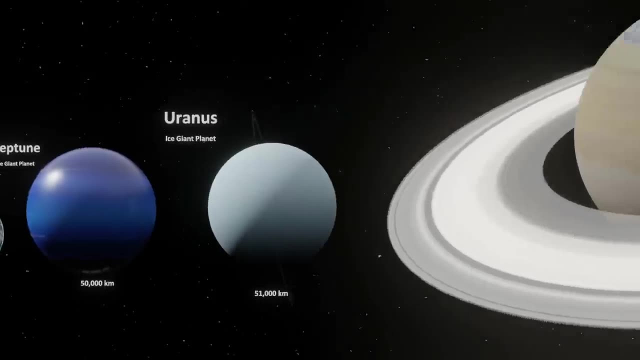 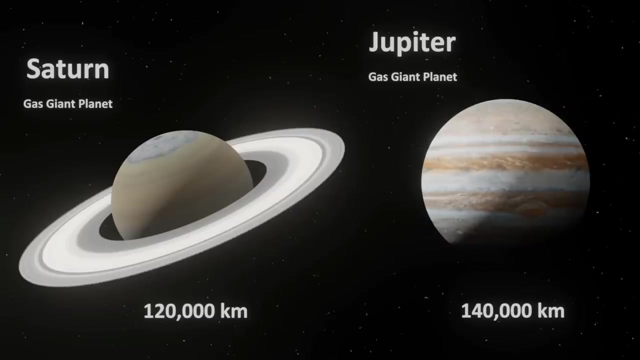 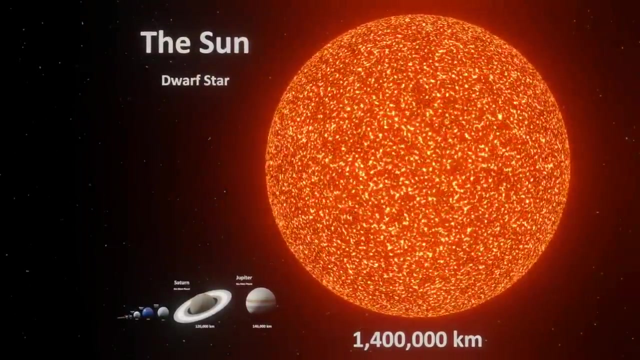 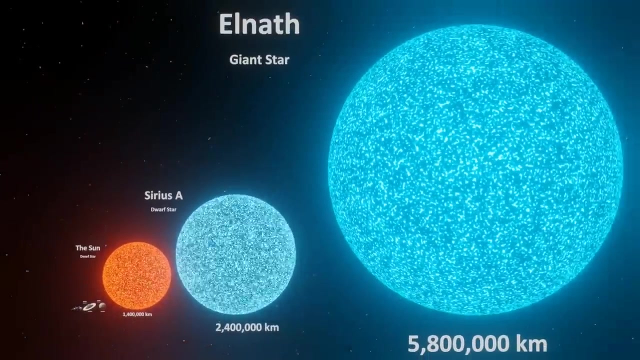 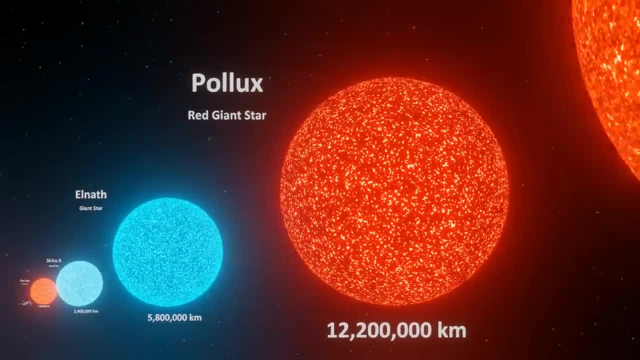 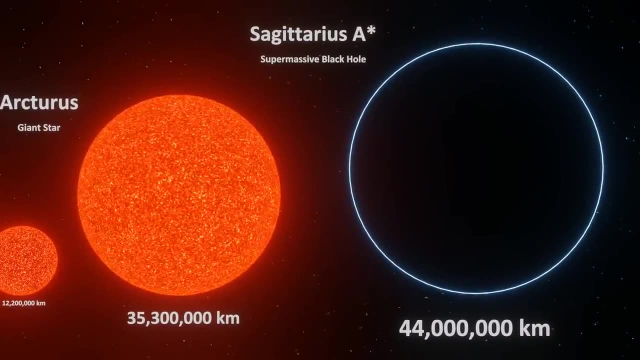 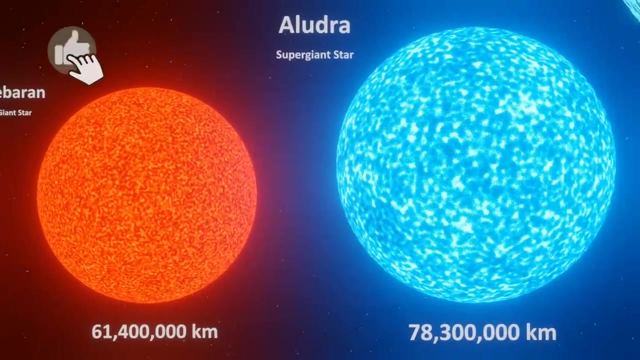 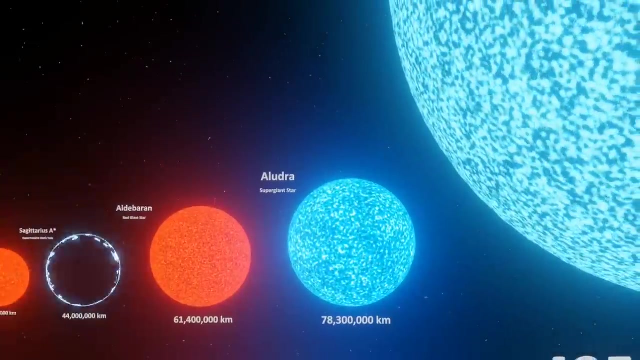 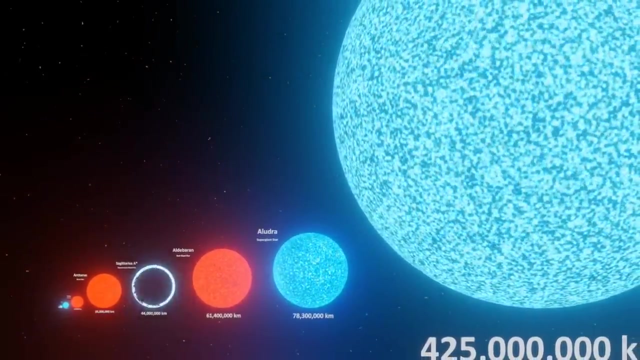 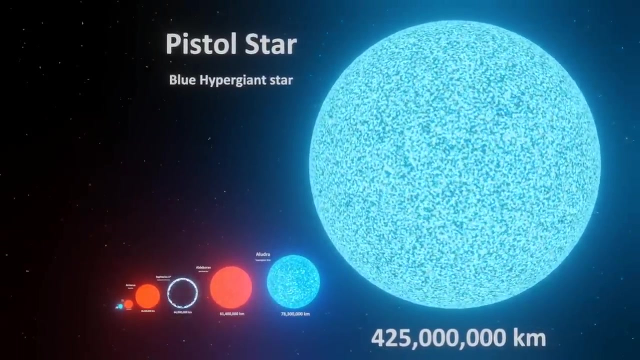 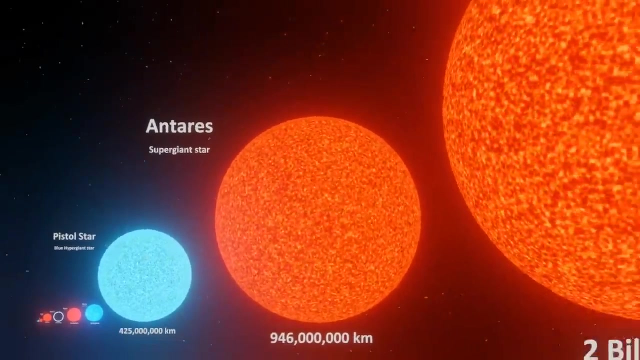 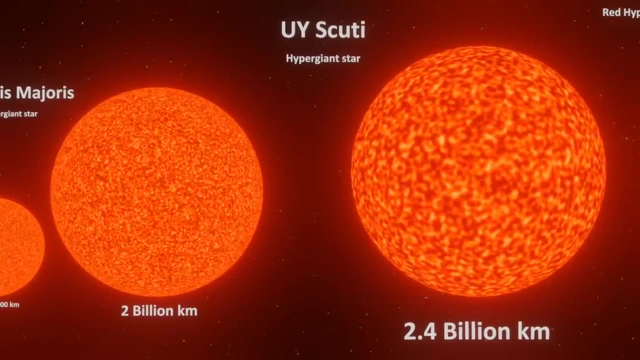 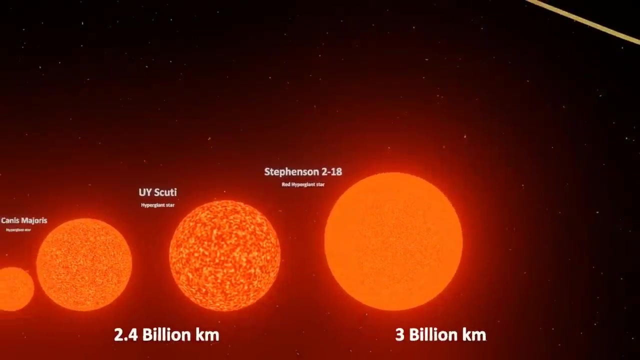 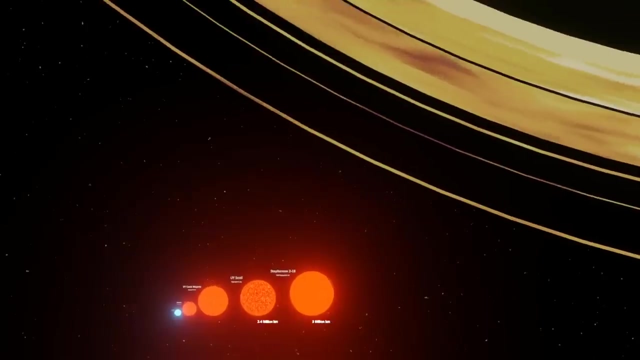 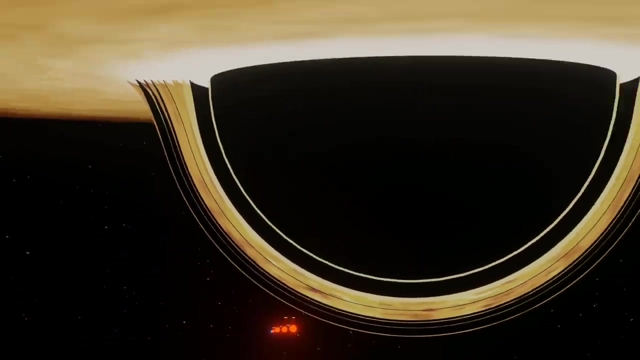 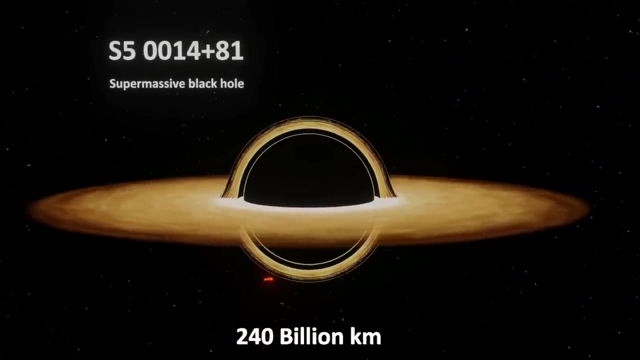 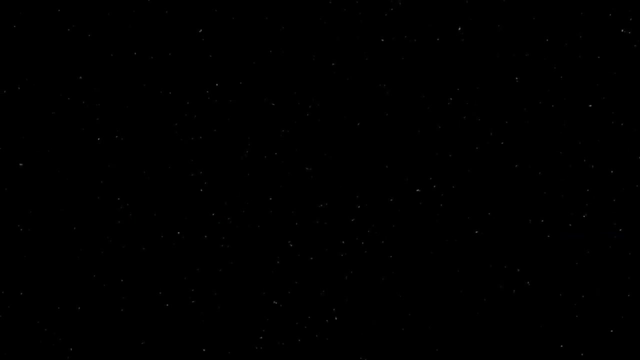 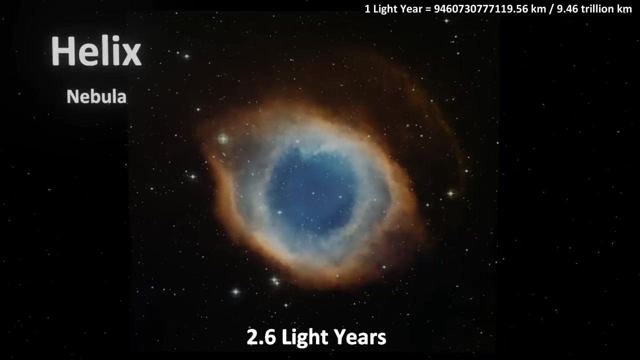 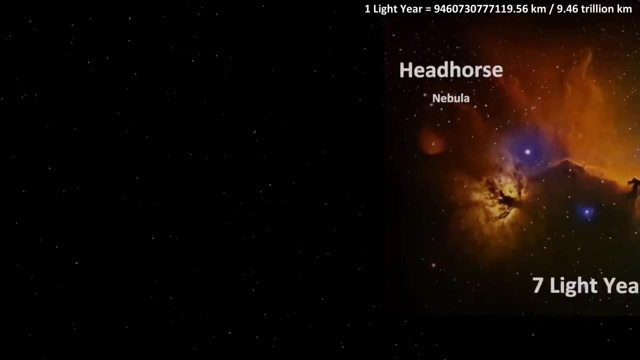 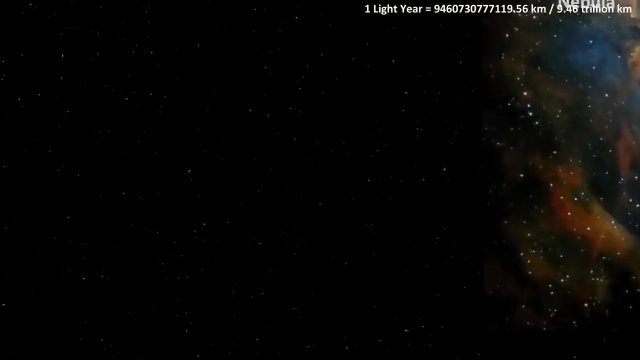 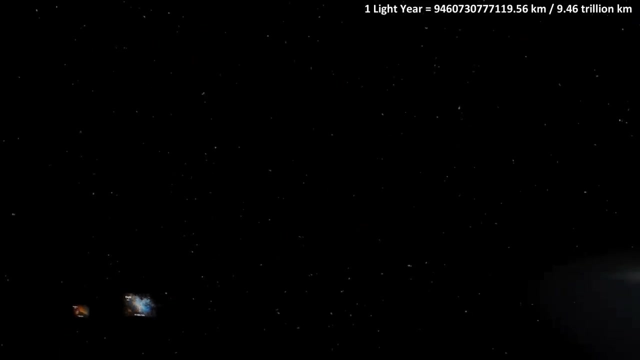 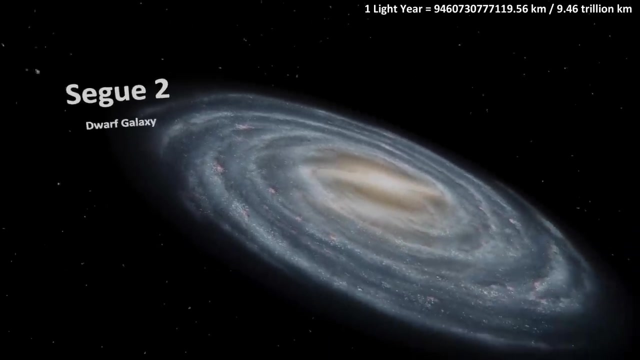 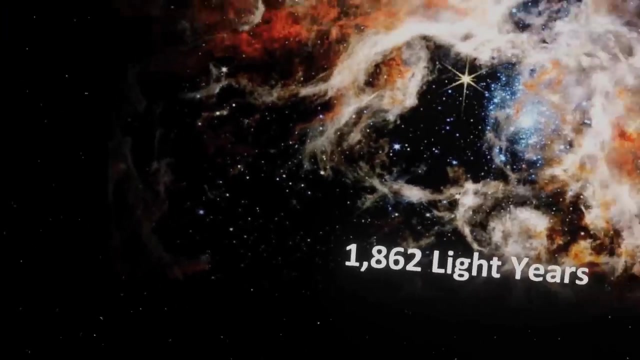 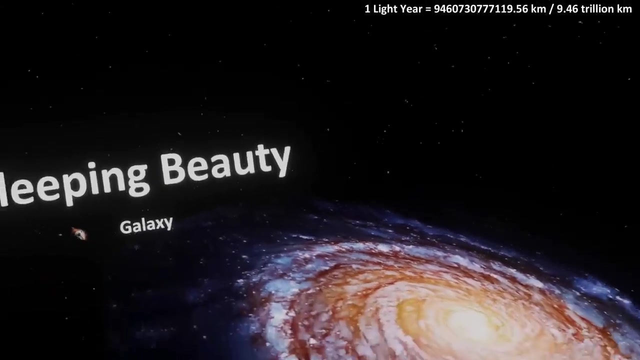 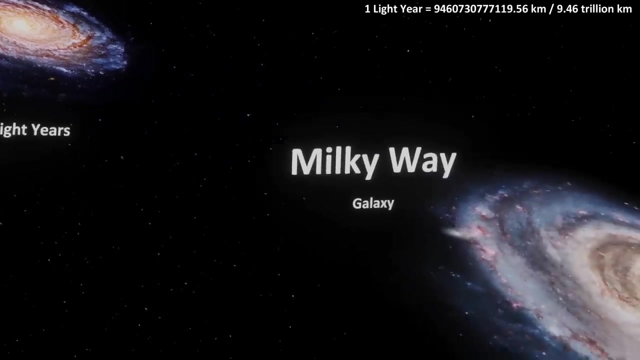 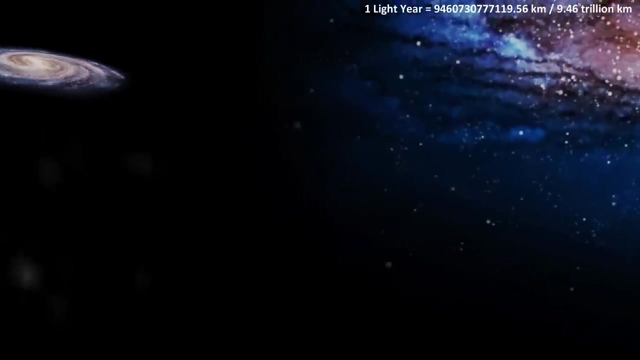 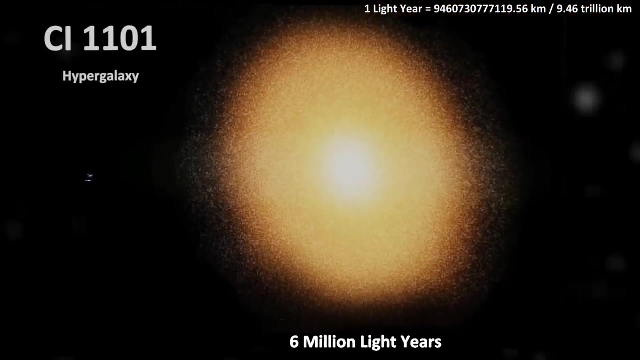 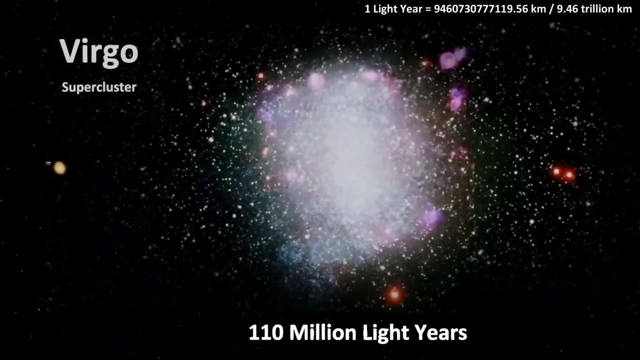 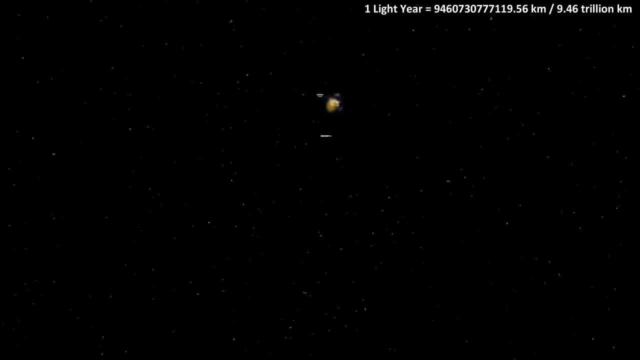 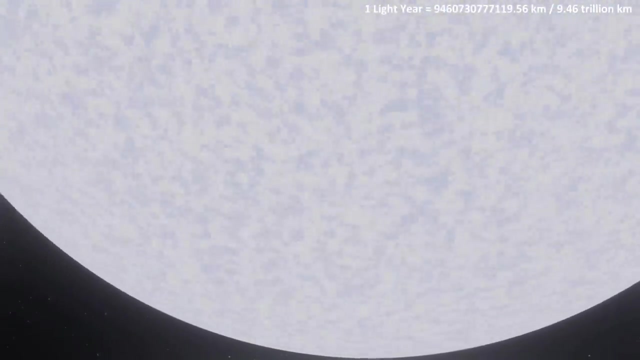 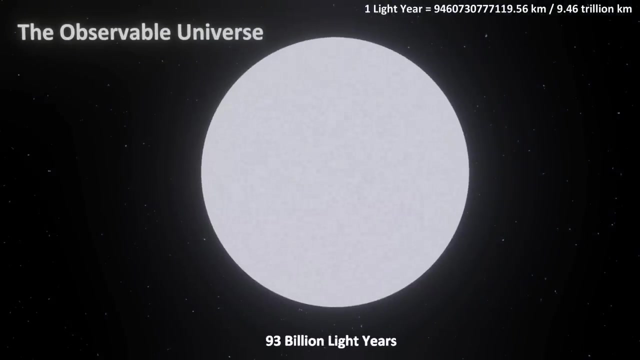 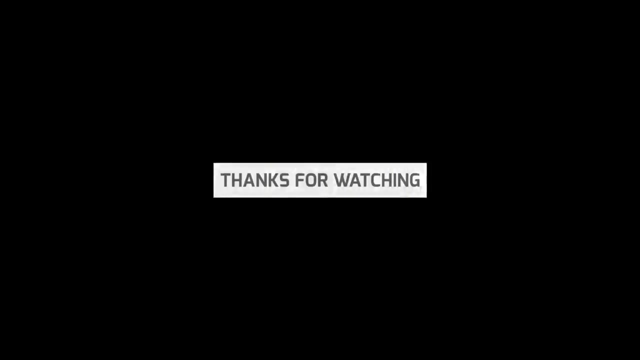